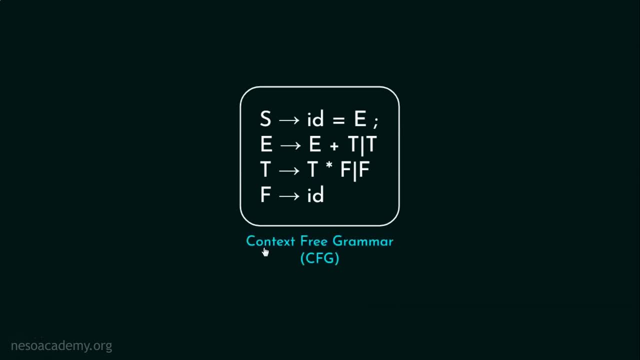 which we have used in the syntax analysis phase is called the Context-Free Grammar, or CFG. Observe, this is called grammar. Now, this one is a bit different from the grammar of natural languages like English. This is the grammar of formal languages. 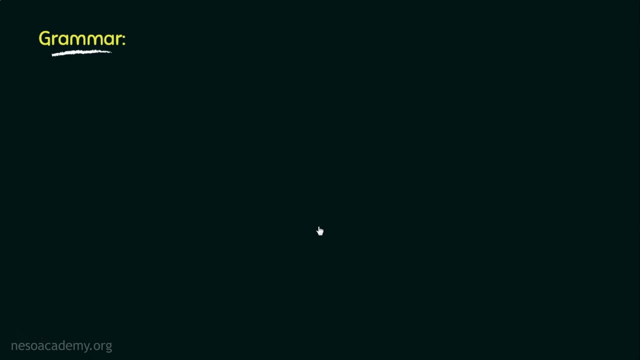 Let me illustrate. Let's take a grammatically correct English sentence: learners are awesome. Well, indeed, you all are. Now observe the sentence Here. the sentence has three words: learners are and awesome, And it is written in this particular order, Replacing the noun learners. 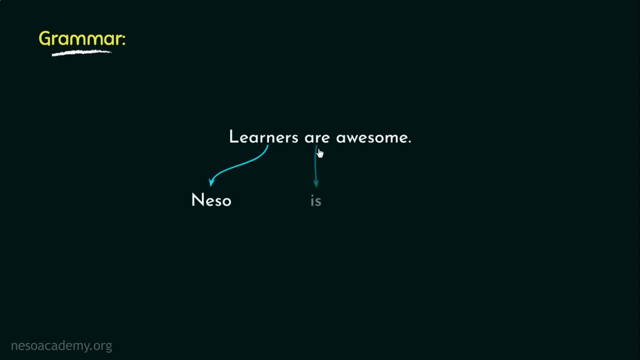 by another noun, say neso, the verb are by is. there is another verb and the adjective also Awesome, by good, which is another adjective, we get another grammatically correct English sentence: Neso is good. Well, I hope that's what you feel about us. 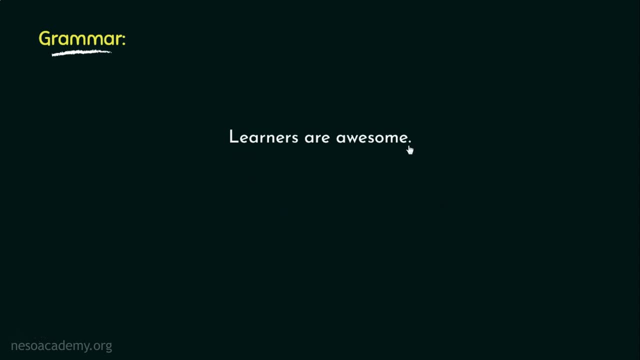 So the structure of the sentence- Learners are awesome- can be stated as Noun, then Verb and thereafter Adjective, Now Verb and Adjective form the Verb Phrase, And Noun and Verb Phrase in this particular instance is forming the sentence. Now, generally, these Noun, Verb, Adjective, Verb, Phrase Sentence are called the Variables. 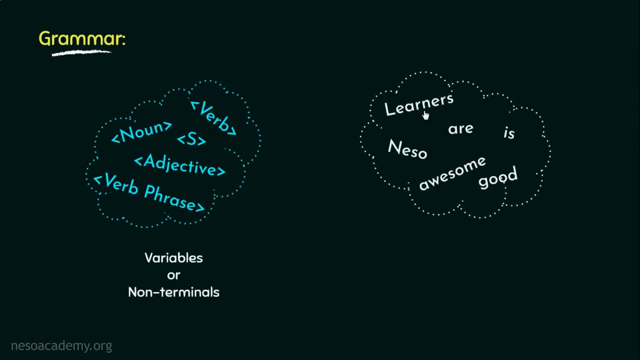 or Non-Terminals. Whereas the words Learners, Neso Are Is Awesome and Good, these are called the Constants or Terminals. Now why is so? Let me explain. Consider this particular structure: Noun followed by Verb, followed by Adjective. 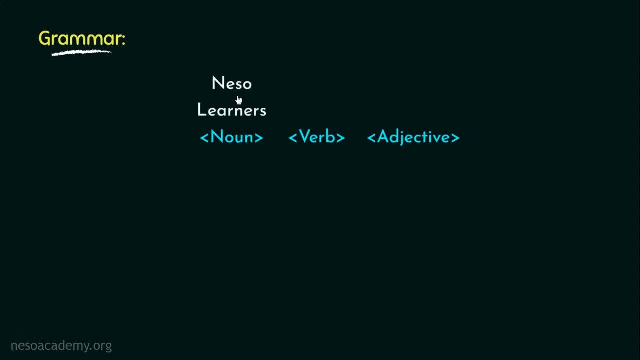 Now for Noun. we have two options: Learners and Neso. Now, once we select Learners from the available choices for the place of Noun, it is fixed. We can't choose anything else now. Similarly for Verb, we have two options: Are and Is. 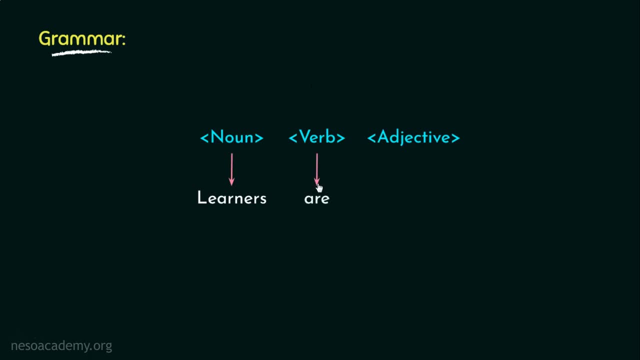 Selecting Are for the verb's position means we have made up our minds, and now Are's been fixed for the verb's position. Then again for Adjective. We have two more options: Awesome and Good. Let's select Awesome, and now the Adjective's position has also been fixed. 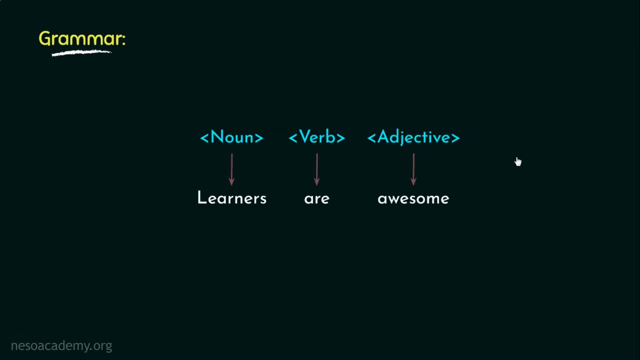 We can't undo that, Basically, when the structure had these, that is, the Variables or Non-Terminals, we had options to choose from. That's why these are termed as Variables. Contrarily, once we generate the sentence, Learners are Awesome. 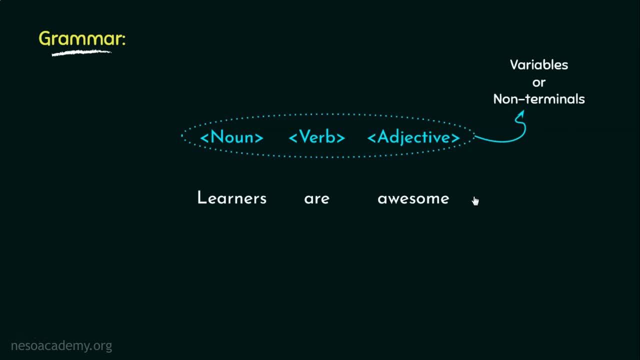 So why are we terminating the places of these? Basically, we are terminating the generation process, And that's why these are called Constants or Terminals. So, since these are terminating the process of generation, that's why these are called Terminals or Constants. 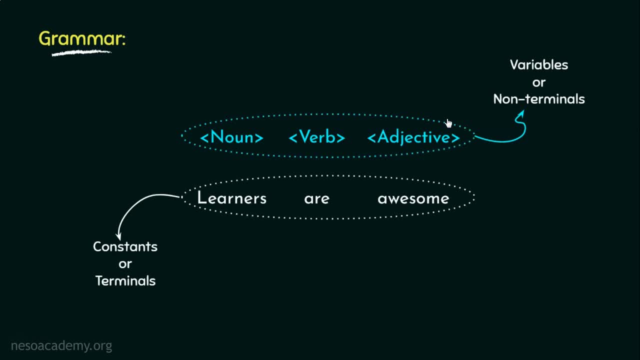 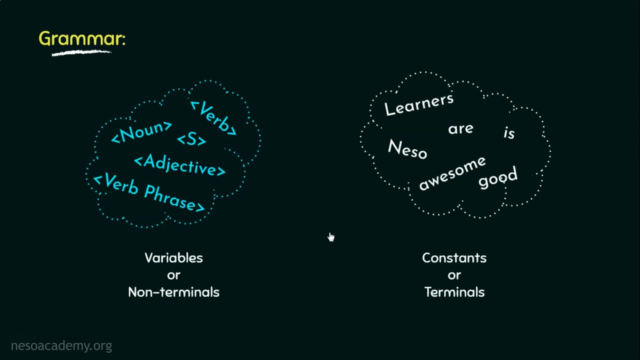 And since these give us the options to choose from, and also these don't terminate the generation process, that's why these are being called Non-Terminals or Variables, because the outcome may vary Based on what we choose. Now, coming back to our discussion of Grammars, we have the set of Non-Terminals in one hand. 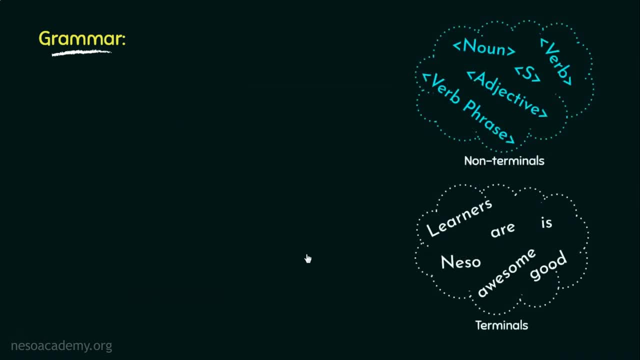 and the set of Terminals on the other hand. Now let's recall the generation process. for this specific instance, Sentence can be rewritten as Noun, followed by Verb Phrase. Then again, the Verb Phrase can be rewritten as Verb, followed by Adjective. Now, Noun can be rewritten as either Learners or Adjectives. 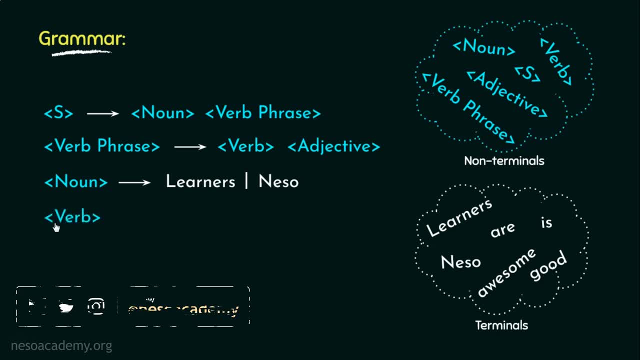 Similarly, Verb can be rewritten as either Are or Is. Finally, Adjective here can be rewritten as either Awesome or Good. Now, if our vocabulary is restricted to Learners, Nesso Is: Are Awesome and Good. that is, these words only. 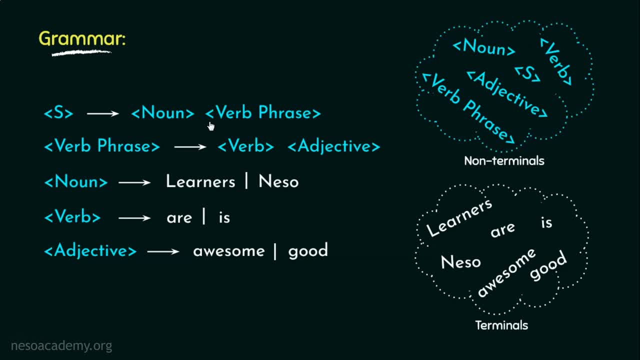 And our sentences are only of the form Noun followed by Verb Phrase, and Verb Phrase is Verb followed by Adjective. Then we can describe the formal grammar using four tuples: N, T, P and S, Where N denotes this collection of Non-Terminals, T specifies this particular collection of. 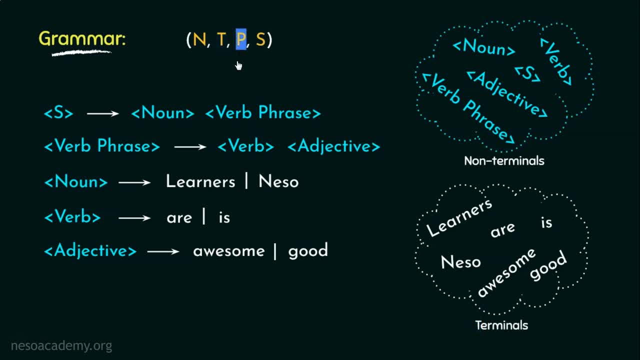 Terminals, thereafter P, is this specific set of rules which will help in the production of sentences, which is nothing but the strings of Terminals. like Learners are Awesome. Finally, S denotes this variable. This is the variable sentence in here which will start the derivation of sentences. 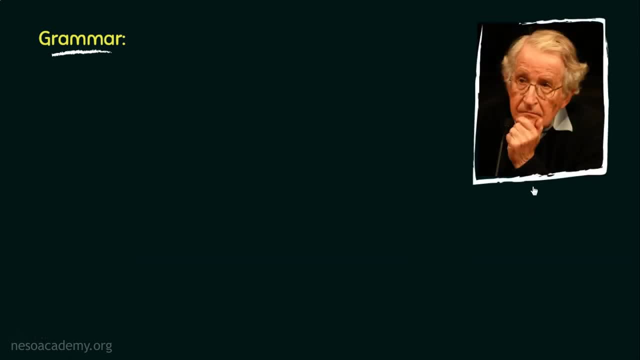 Now, in the year 1956, this genius linguist, Avram Noam Chomsky, gave a formal definition of grammar. There he stated: A phrase structure grammar, which means a generative grammar, ie a grammar which generates, or simply grammar, is N T P S. 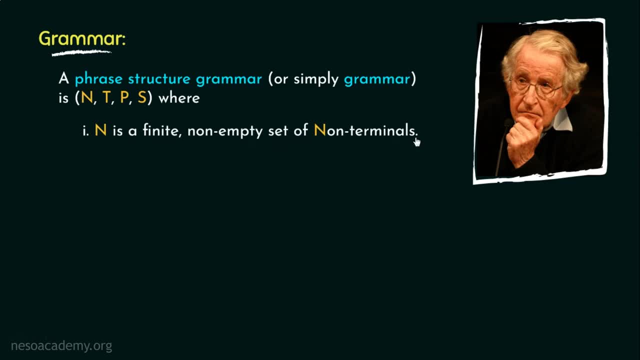 Where N is a finite, non-empty set of Nouns, That is, the collection of non-terminals, should be finite because, since it is a grammar of a language, naturally it should be finite. Also, it should not be empty, because if it is empty we won't be able to generate the 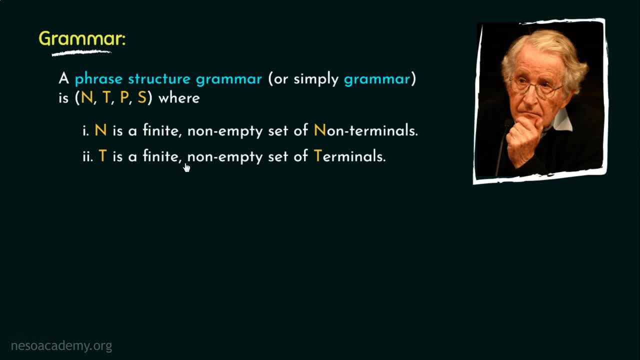 terminals, Then T is a finite, non-empty set of terminals. Here also the terms finite and non-empty are specified for the same reasons. Now, if section T will result in Phi, that is, the set of non-terminals and the set of terminals are two disjoint sets and don't have anything in common. 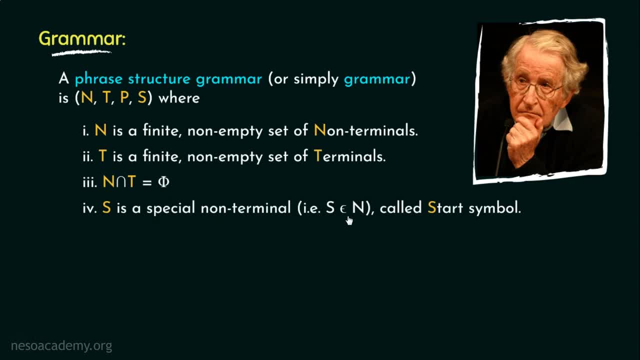 Now, S is a spatial non-terminal, That is, S belongs to the set of non-terminals which is called the start symbol. Now, why it is called start symbol? Because from S the process of derivation will initiate. Finally, P is a finite set whose elements are of the form. 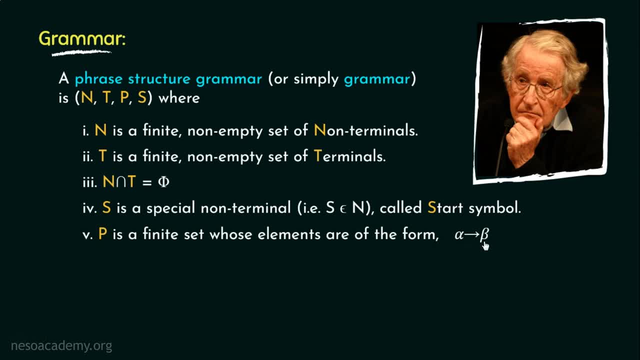 P is a finite set whose elements are of the form. P is a finite set whose elements are of the form Alpha can be rewritten as beta, where alpha and beta are the strings over N union T, Meaning they may be a mixture of non-terminals and terminals, or only non-terminals, or only. 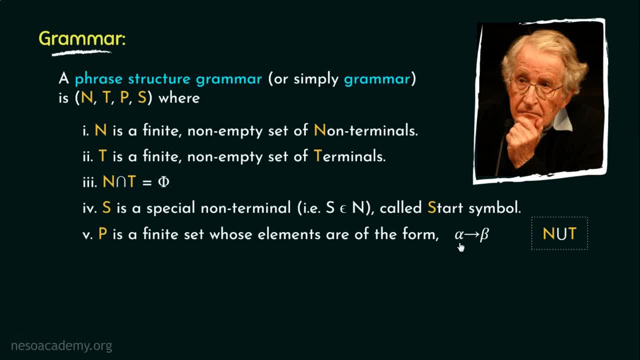 terminals. Nevertheless, alpha must have at least one non-terminal, because we already have seen, without a non-terminal we cannot generate anything. And also, the elements of P are called production rules. By the way, for your information, way before Chomsky, probably in the 6th to 5th BCE, the 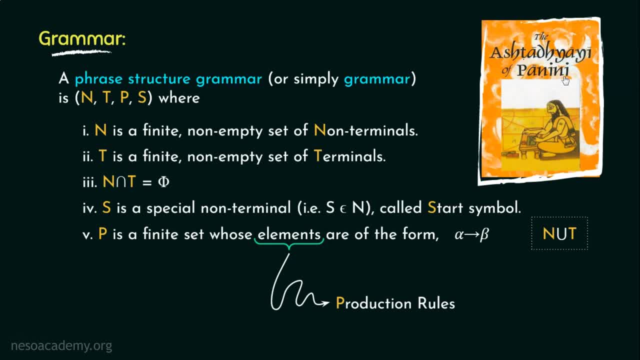 ancient Indian grammarian, Panini, used formal production rules and definitions in order to describe the formal grammar of Sanskrit in his noble work Astadhyayi ie Ast-Adhyayis, or Eight Chapters. Now I believe you all have the proper understanding of the meaning of these words.